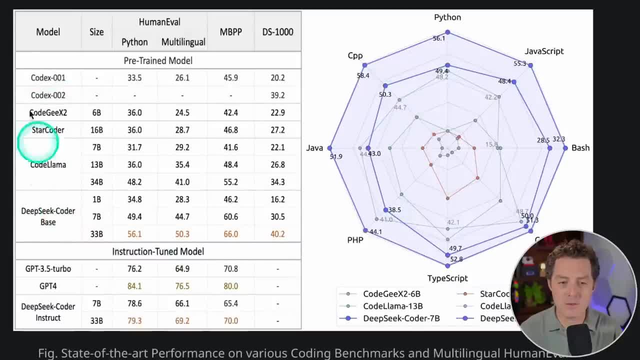 Deepsea Coder Base performs better than any other open source model on this list. Now, the one that they did not mention is the FIND model P-H-I-N-D, And I'm going to be testing that in a separate video And here it is. against the closed source models, It beats GPT-3.5 Turbo. 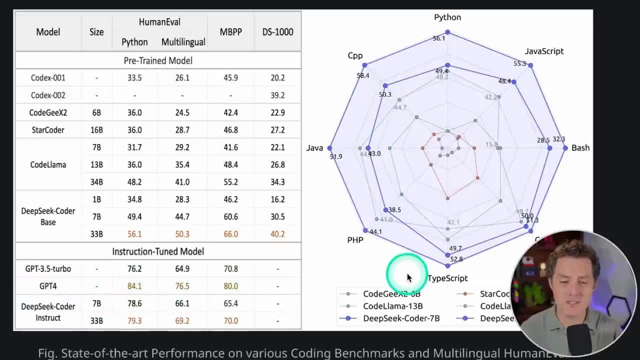 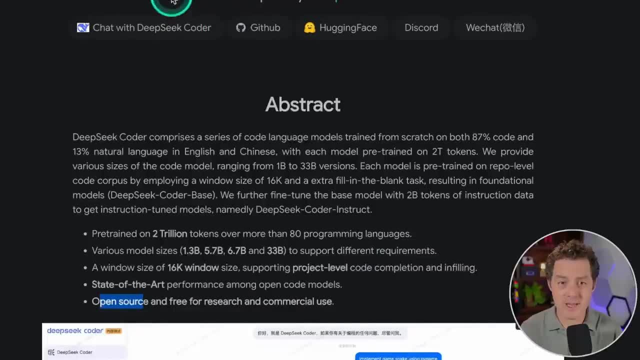 and it gets really close to GPT-4 in performance. All right, enough talk, Let's test it. So I'm just going to go ahead and test it through the website itself And all you need to do is sign up for an account and you can test it. But again, this model is completely open source You 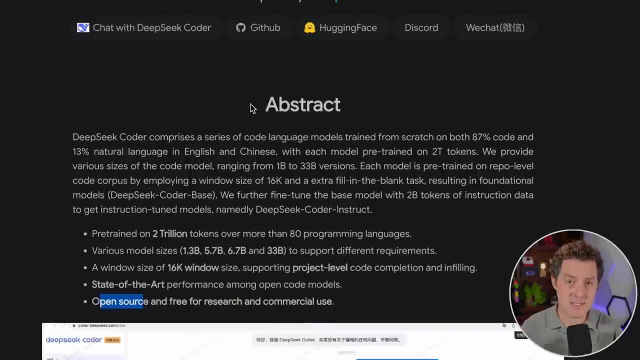 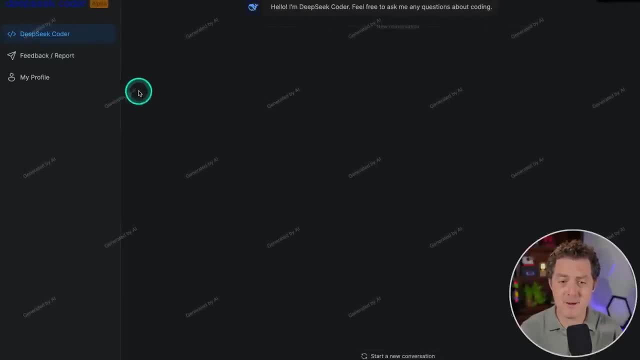 can use one of the many methods that I've shown in previous videos for how to get this loaded on RunPod or locally on your computer. So I've already signed up. Here it is, And it has this pretty hideous background generated by AI. So that's really cool that it was generated by AI. 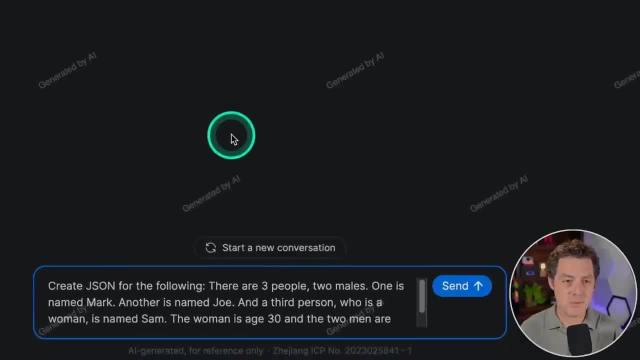 but, geez, this background is very ugly. All right, the first test that we're going to run is one that we've actually used on every other test that we've run on our original LLM rubric. So create JSON for the following: 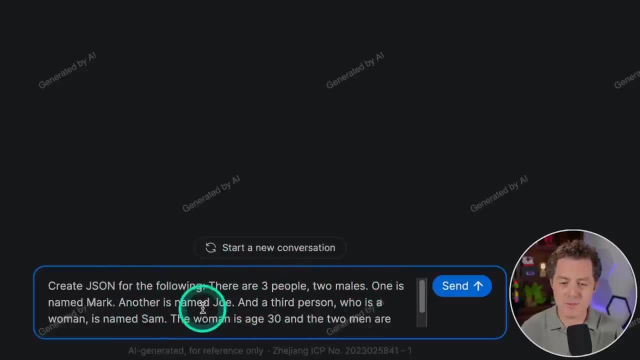 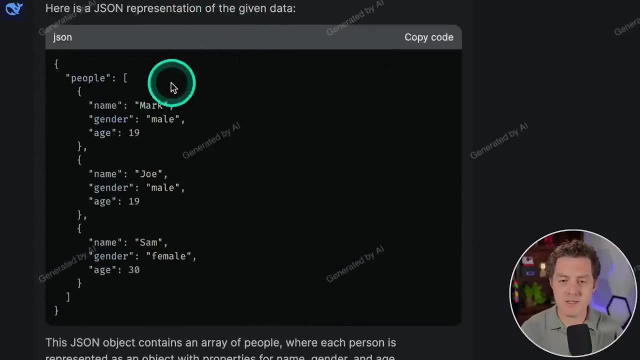 All right, let's see. Here's the JSON representation of the given data. So we have people: name, name name, gender and age. Perfect, Yeah, that's an absolute pass, And I'm going to start a new conversation each time so that it doesn't have any memory from the previous. 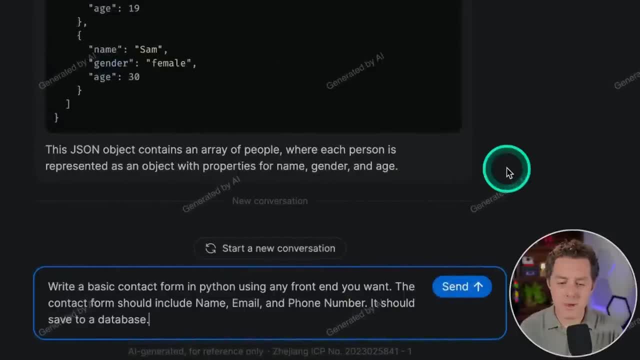 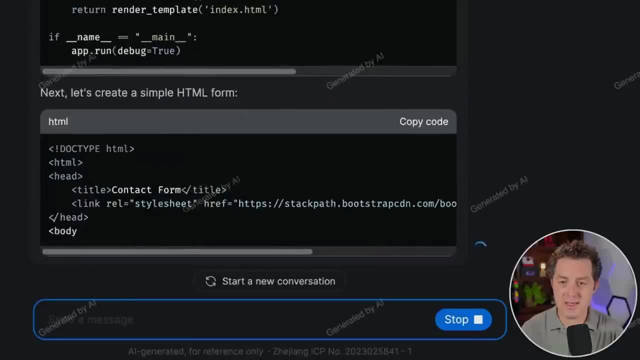 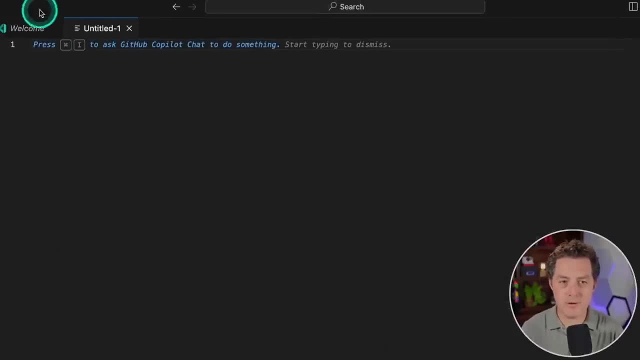 code. already It looks like it's going to use Flask and SQLite. All right, here's the entire Python section, So let's go ahead and copy that. Switching over to Visual Studio Code, I'm going to open a new window. I'm going to open a new tab. paste in the Python code It already recognizes. 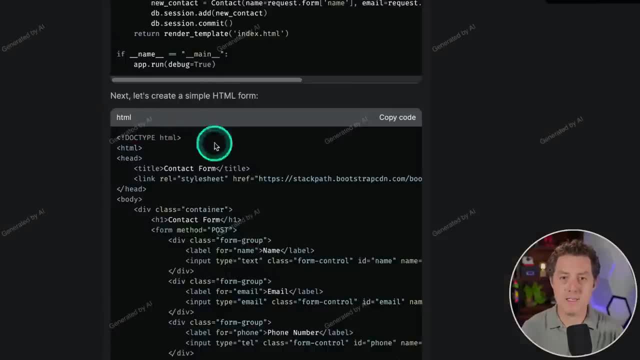 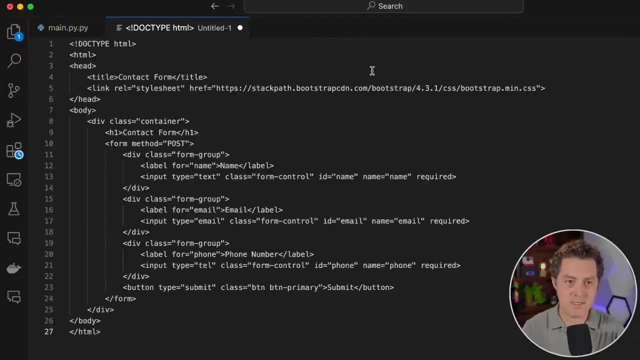 its Python as mainpy. Then we have a second HTML which is going to be the front end, So I'm going to go ahead and copy the code there. Switch back to Visual Studio Code. I'm going to create a new file, I'm going to paste in the HTML and I saved it as formhtml And it actually says: save this. 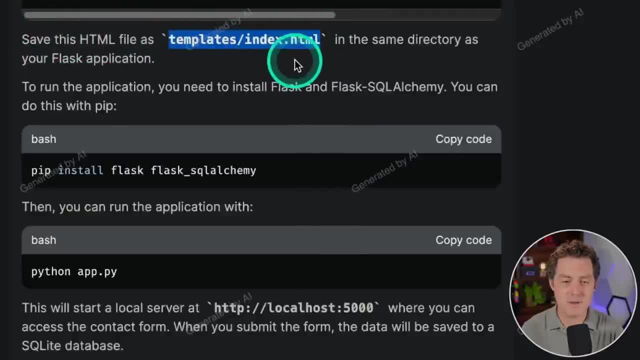 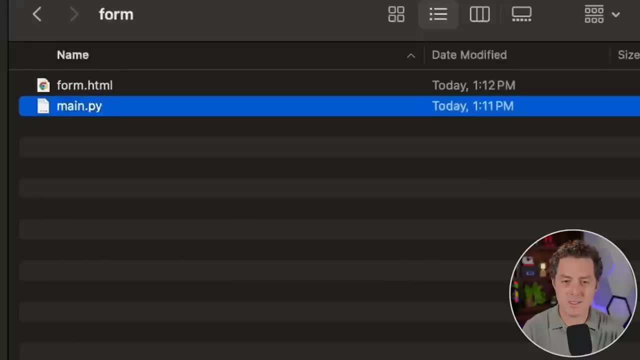 HTML file as templates slash indexhtml. So I actually need to change that. I'm going to change a couple of things here. So it says mainpypy. Obviously that's wrong. I'm going to go ahead and remove that. secondpy. I'm going to create a new folder called templates And then I'm going to 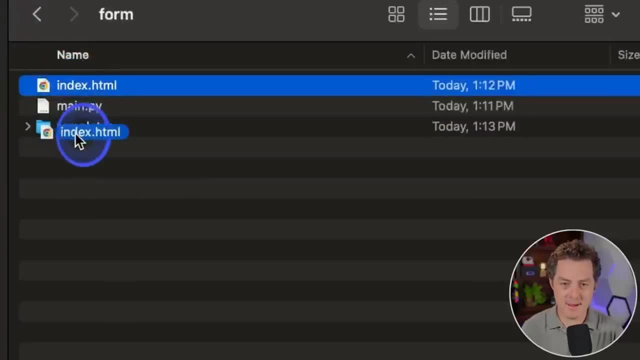 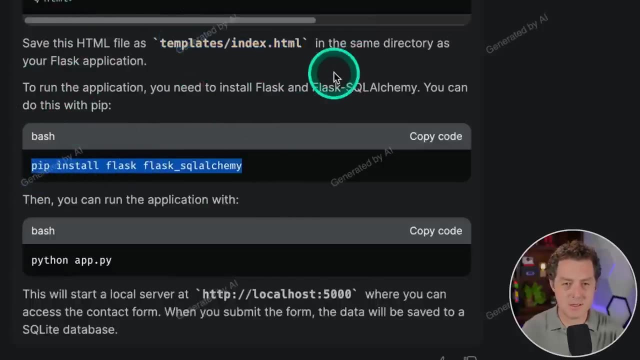 name this indexhtml and put that in templates. There we go. Now back to DeepSeq. It says: to run the application you will need to install Flask. So let's go ahead and copy this code and install it. Switch back to Visual Studio Code. Let's open up the terminal. Let's go ahead and spin up a. 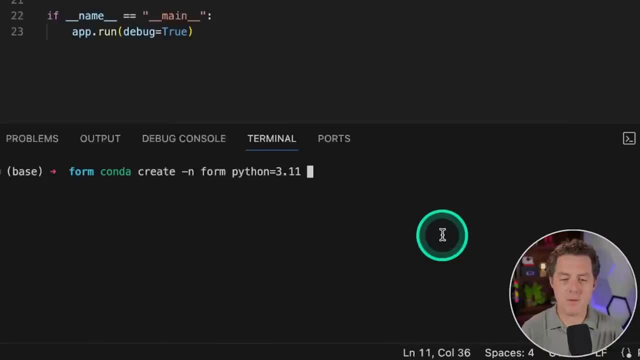 conda environment. conda create dash n form. Python equals 3.11.. All right, then we're going to activate conda. conda activate form. Okay, we're in form now. Now I'm going to try installing it. 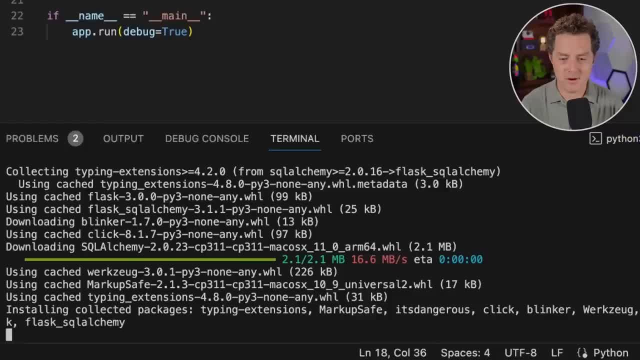 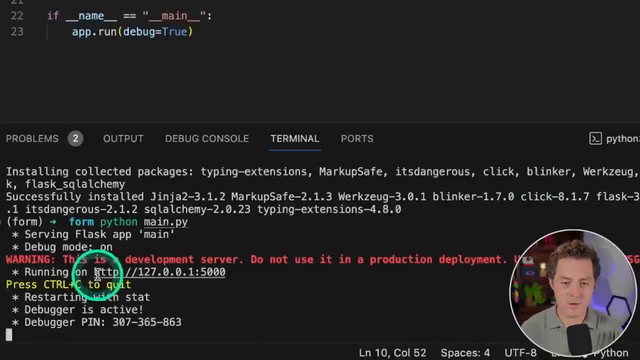 using Python from the folder. I know it's already in. All right, there, it looks like it's working, And then we're going to run python apppy. All right, it looks like we got it up and running now, So running on. let's open it up And there we go. We got a contact form with name: email. 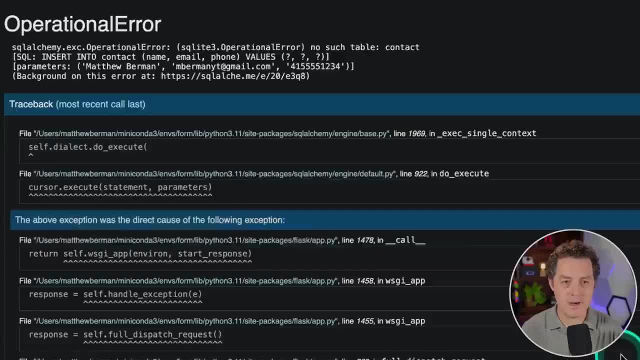 and phone number And I filled it out. Let's click submit. Oh, we got an error. No such table contact, And I guess this makes sense because we never actually created the table. So let's try to get it to do that. All right, so I'm just going to type: when submitting this form, I get this error. 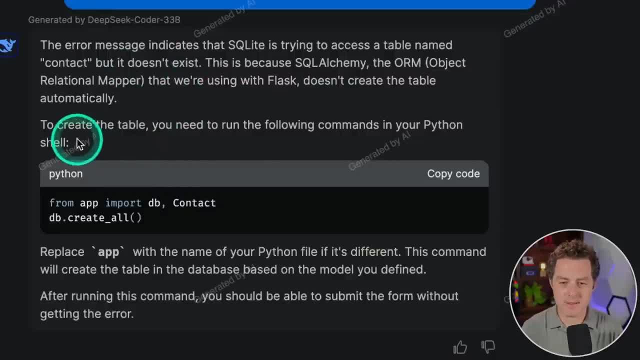 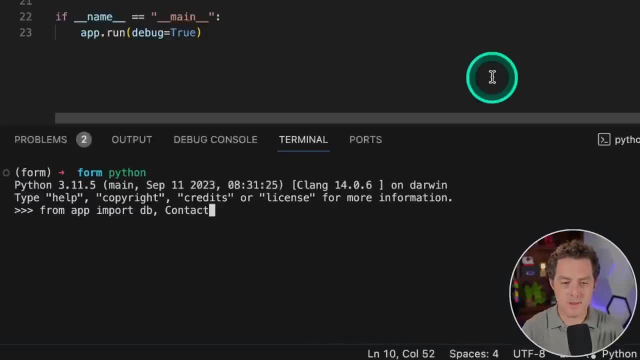 and I paste it in the air. Yep, And it says it doesn't create the table automatically. So to create the table you need to run the following commands in your Python shell. So let's go ahead and do that. So let's open up Python. Then we're going to do from app import, DB contact: no module. 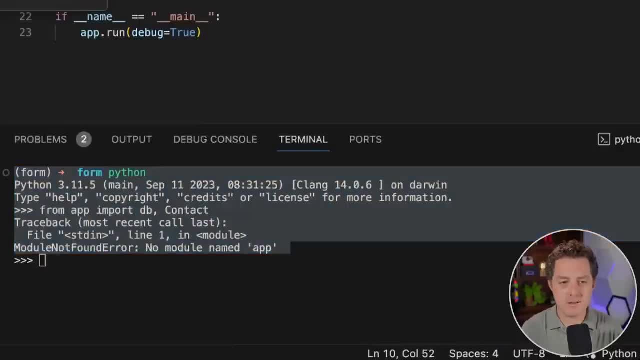 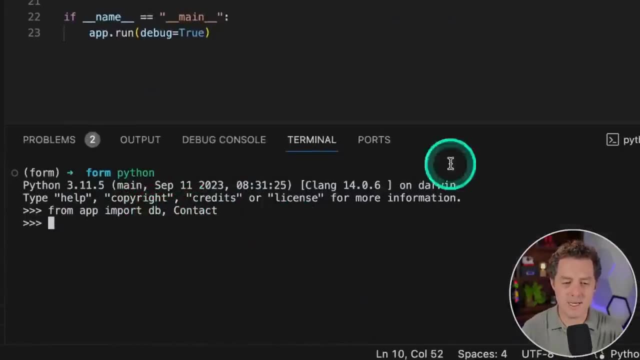 named app. Ah right, because I named it mainpy. Let's go ahead and rename this file apppy. And let's try again From app import, DB, comma, contact. And that worked, And now we're going to create all from the DB. So 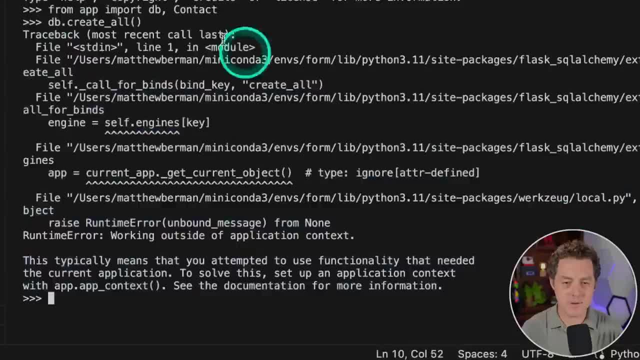 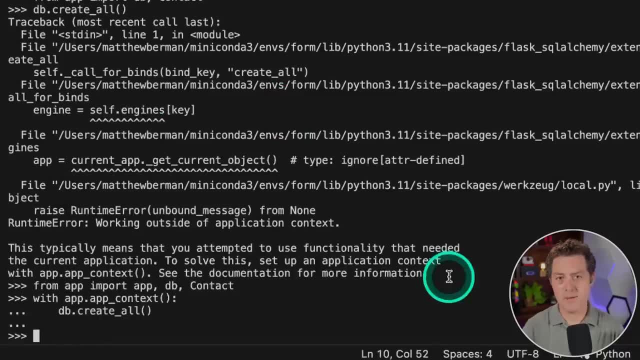 dbcreate, underscore all and then parentheses. Looks like we ran into another issue, So I'm going to copy these logs and paste it back into the app and see what it says. All right, let's try that. Okay, maybe that works. Let's try. Here we go. Python apppy. Let's open it up. Here it. 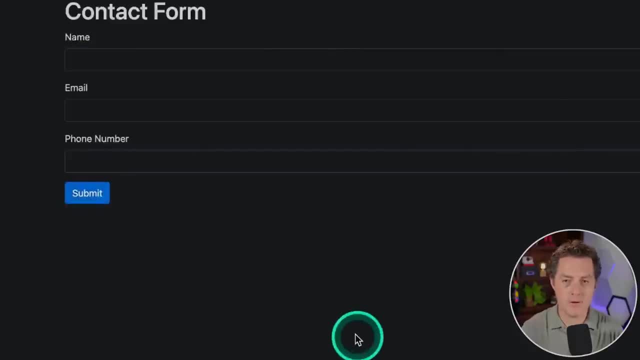 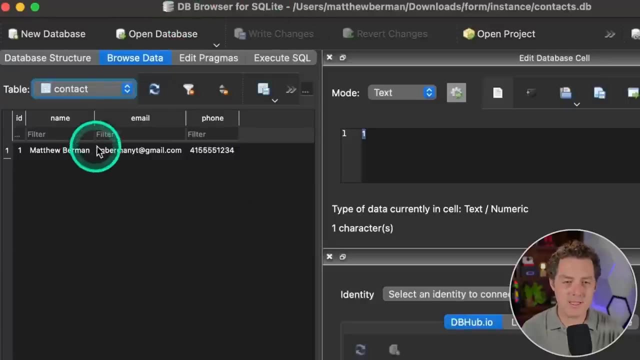 is. I'm going to input some information and submit. Okay, I think that might have worked. I think it inserted into the database successfully. All right, there it is. I opened up the DB browser for sqlite And there's the information right there. That's what I just submitted, So that. 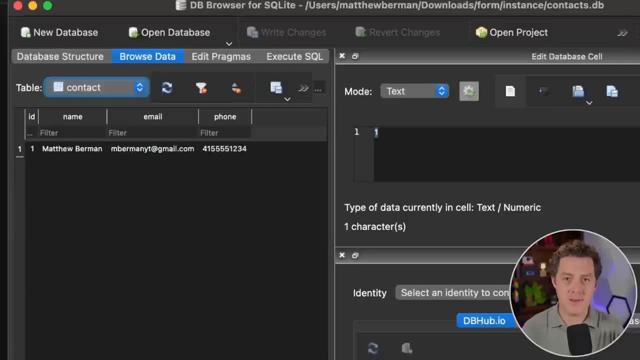 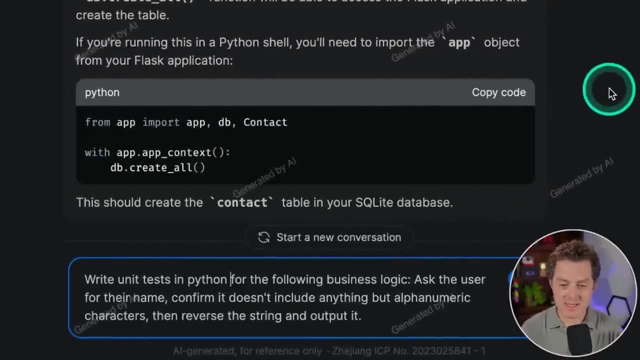 worked. a couple of issues, but pretty minor overall And really the code worked. It was just the fact that I didn't have the database created, So I'm going to give this a pass. Next, write unit tests in Python for the following business logic: Ask the user for their name. confirm it doesn't. 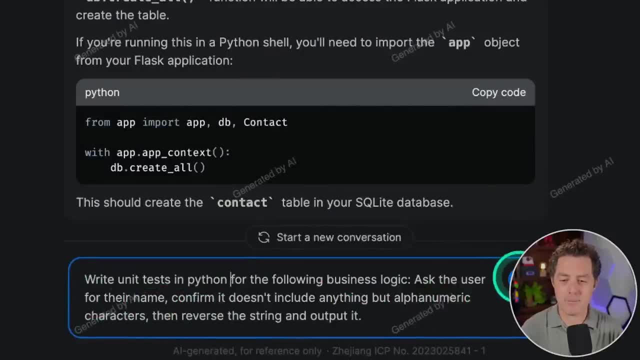 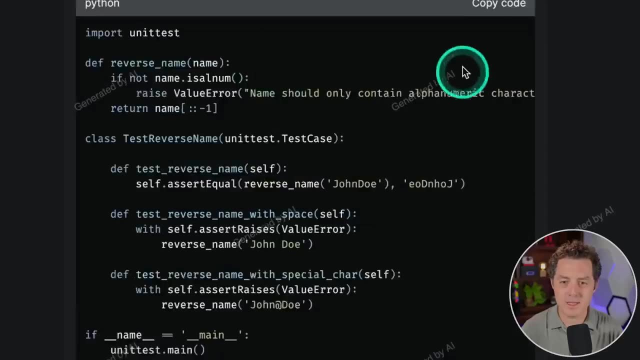 include anything but alphanumeric characters, then reverse the string and output it All right. here's the unit tests using the unit test library, And it also gave me a description of everything, So let's test it out. Copy the code: Okay, so it wrote unit tests, But now how do I actually tell? 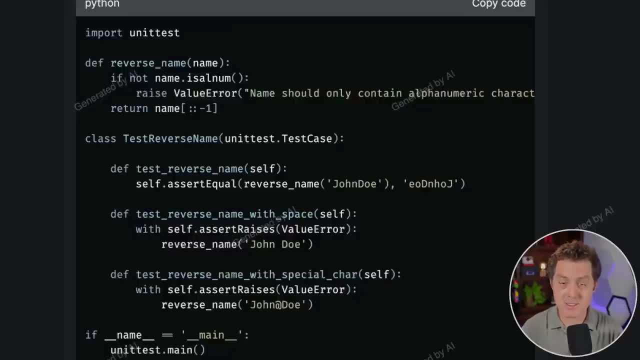 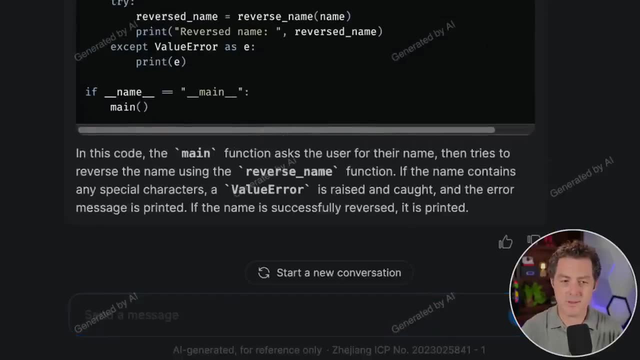 that the unit tests are working. I'm going to have it write code that completes the unit tests and I'm going to test it myself. So now write code that passes all of the tests you just wrote. All right, there it goes. Let's copy this code. switch over to Visual Studio Code. Now I have the 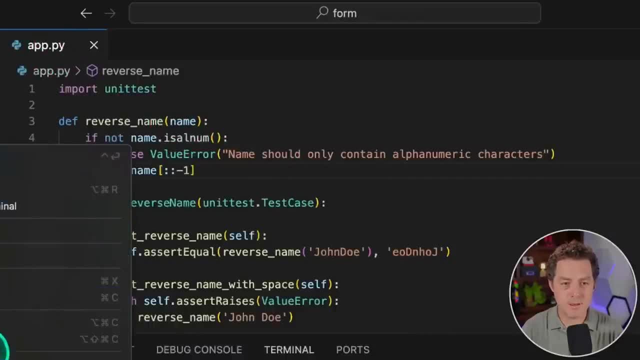 unit tests, and I'm actually going to rename apppy to be testpy, And then I'm going to create a second file, paste the new code in there and I'm going to save it as apppy. Now one thing: I just 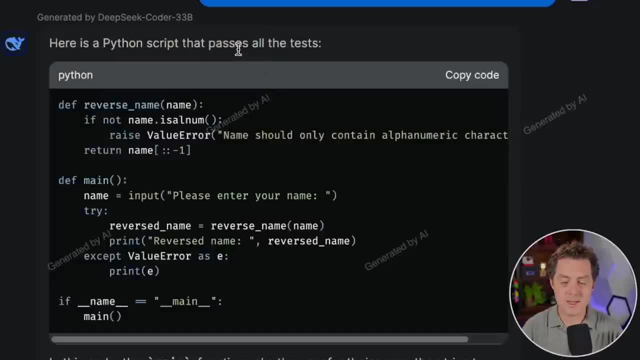 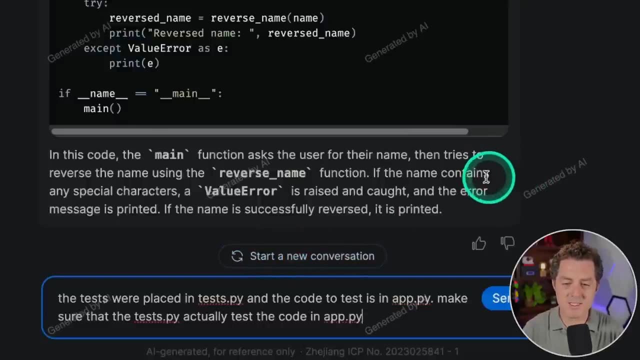 realized is: how is it going to actually test that code? Let's make sure that the tests that we just wrote are related to the apppy file. Okay, the tests were placed in testpy And the code to test is an apppy. Make sure that the testpy is actually testing the code in apppy. Okay, so we 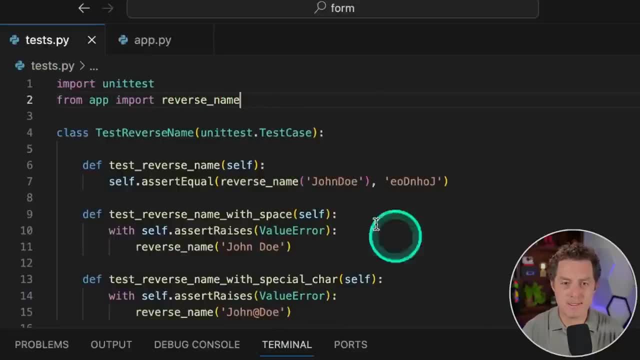 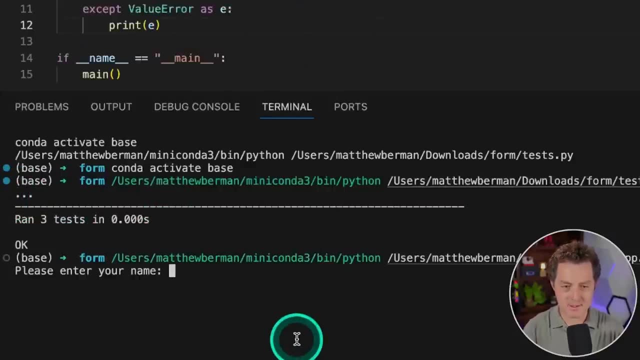 import, reverse name from app And let's give it a test. Okay, looks like we got three passes, So that worked. Now let's just make sure it's working. So I'm going to run the code and see if it actually works. 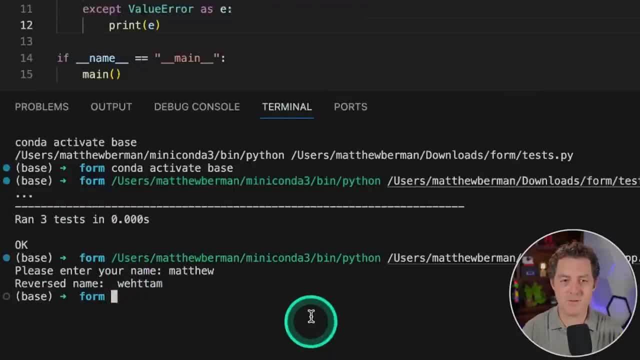 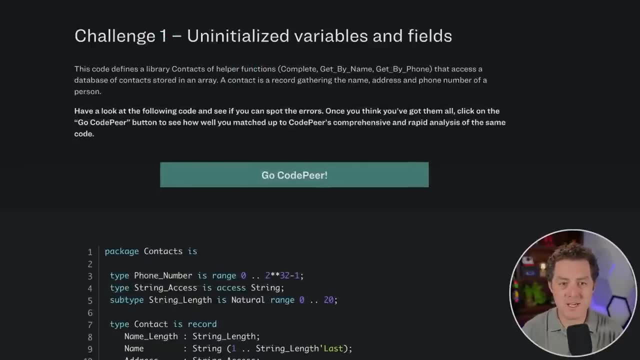 So enter your name, Matthew. there it is. That's my name, reversed, Perfect, And so that's a pass for both the code writing and the code testing. All right. next we're going to use a challenge from the website adecorcom, And 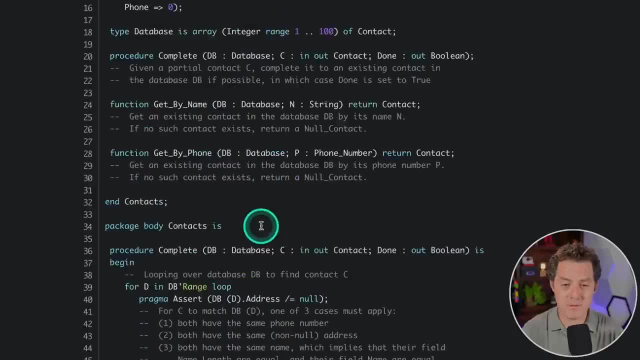 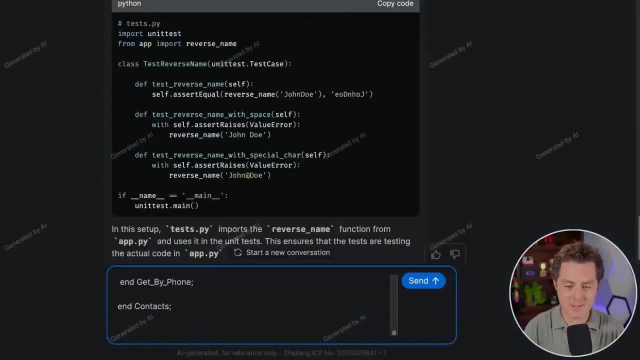 this is a test in which we're going to have the model find bugs in the code. So we have a bunch of code right here. I'm going to highlight it all. I'm going to go to deep sea coder, start a new conversation. I'm going to paste it in And then at the bottom I'm going to say: find all of the. 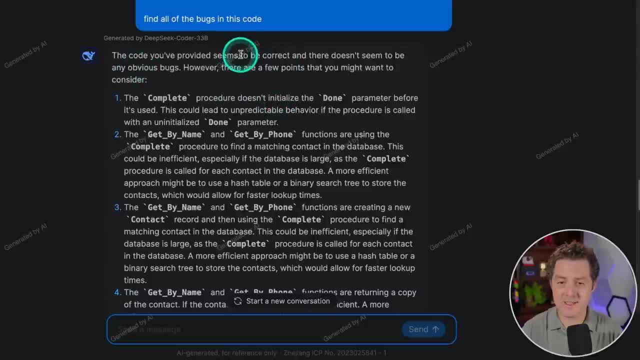 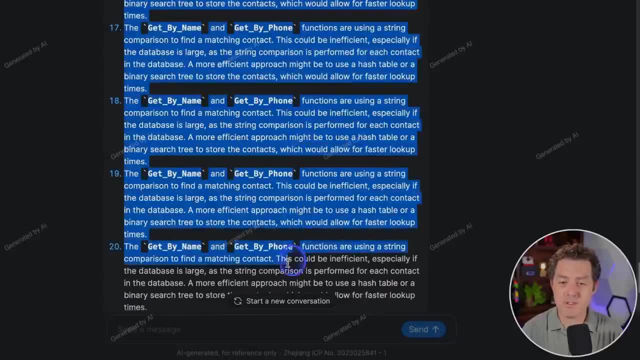 bugs in this code. Okay, so interestingly enough, it says that it seems to be correct And there doesn't seem to be any obvious bugs. However, there are a few points that you might want to consider, And it gives me a bunch of efficiency. 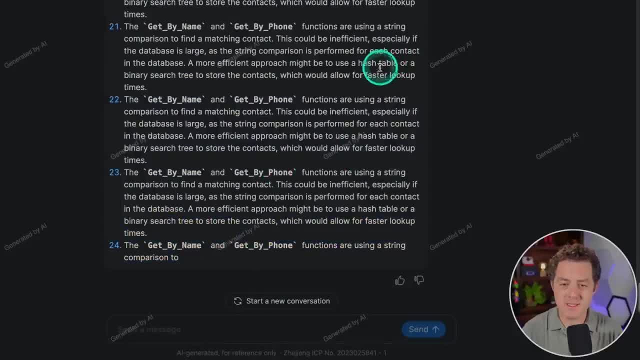 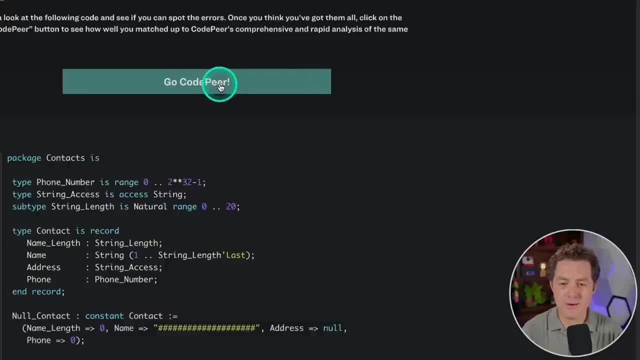 recommendations And then, finally, it just stops. So this is a definite fail, especially because it just seems to output the same thing over and over again. And for those of you who are wondering, when I click go code, peer, we have the errors right there. So I hope this was a good test, but it 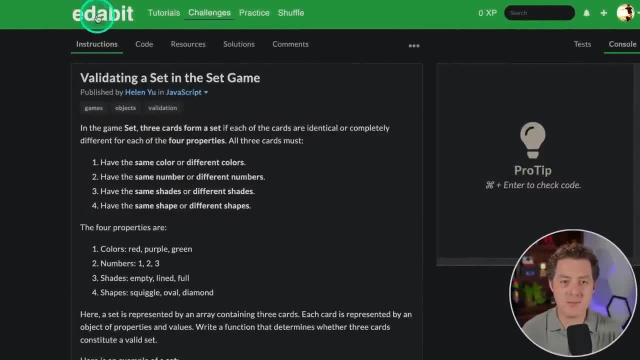 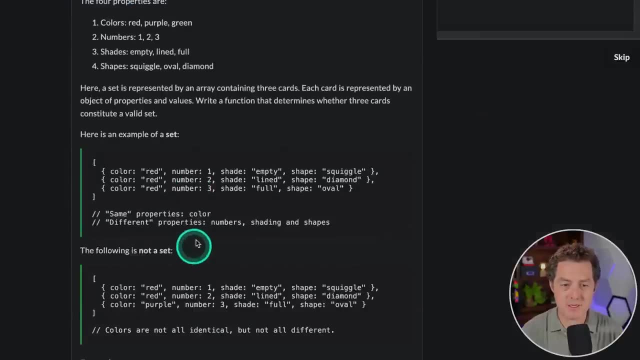 definitely failed. Okay, next we're going to do a coding challenge from the website at a bitcom validating a set in the set game. So we have a detailed description, a bunch of examples, and then we're going to check our code And what the model. 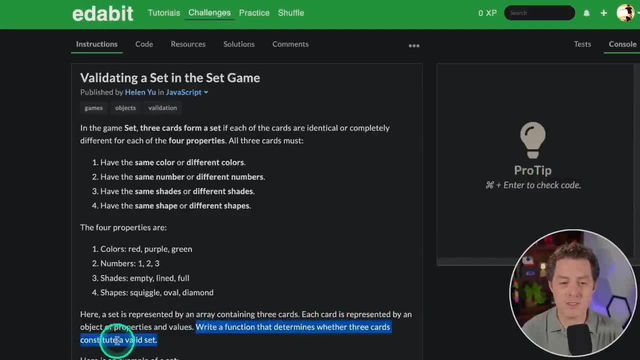 needs to do is, right here, write a function that determines whether three cards constitute a valid set. And all the rules of being a valid set are right here, as well as some examples. So I'm going to copy this whole thing, And I'm just going to copy paste it right into the model. So let's start. 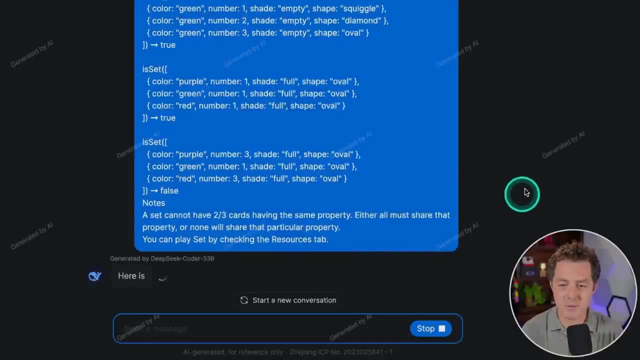 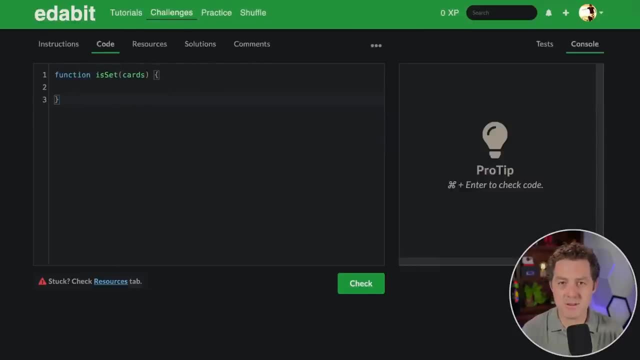 a new conversation paste and then let's go: Okay, that's really short code, But let's see if it works. Okay, back here I realized it's expecting this in JavaScript, So let me do that again And I'm going to specify that it needs to give me JavaScript. So I said: rewrite the code in. 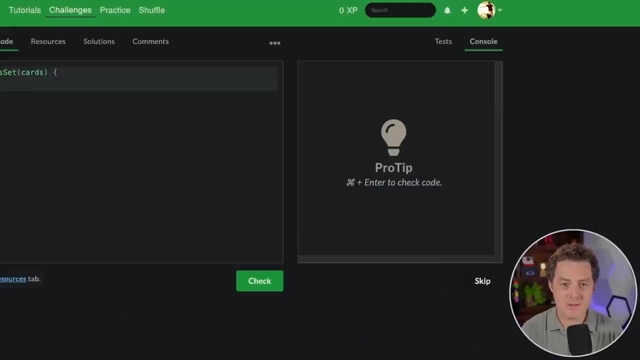 JavaScript. And here we are. Okay, copy code. Let's go back, Let's paste it in and check. All right, test passed. Awesome, Look at that. So that is a pass. All right, next I'm going to have it. 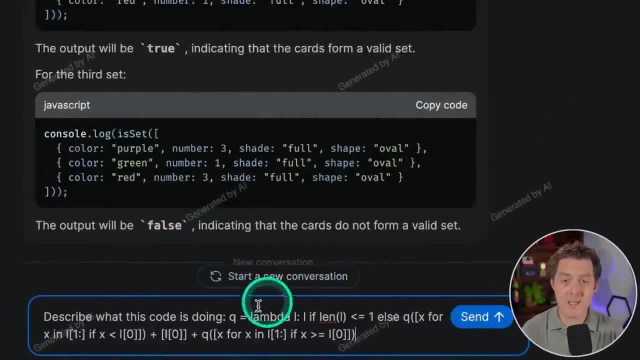 describe what some pretty complex code does, And I've renamed all the variables So it gives no hint as to what it does. But this is a quick sort algorithm So you can see it right here. So I'm going to send. let's see what it does, All right. there it is, So let's see what it does, All right. 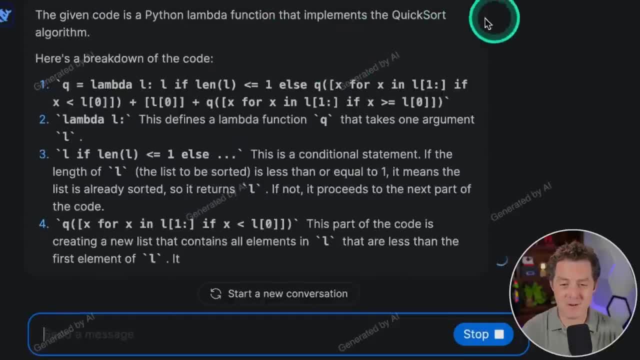 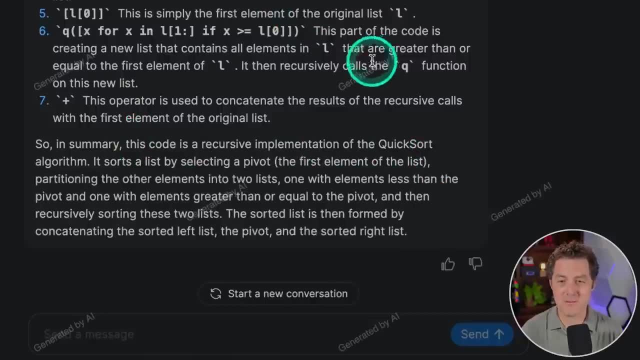 the given code is a Python lambda function that implements the quick sort algorithm. Here's a breakdown of the code. This is extremely impressive. So this code is a recursive implementation of the quick sort algorithm. This is phenomenal. That's an absolute pass, All right.